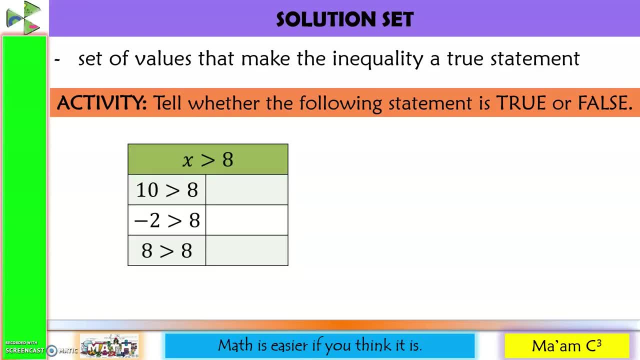 I'll tell you a technique. Do you know the game Pac-Man? Here's the thing. Just remember that Pac-Man eats the bigger number. Pac-Man is going to eat 10.. So it means 10 is greater than 8.. 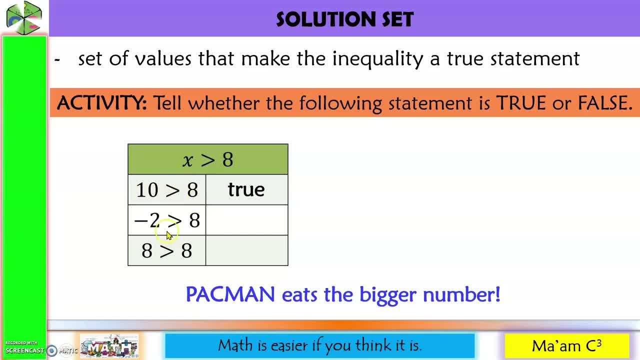 Is that true? Yes, it is. Here Pac-Man is going to eat negative 2.. Is negative 2 greater than 8? No, So this is false. Here Pac-Man is going to eat 8.. Is 8 greater than 8? No, They are equal. 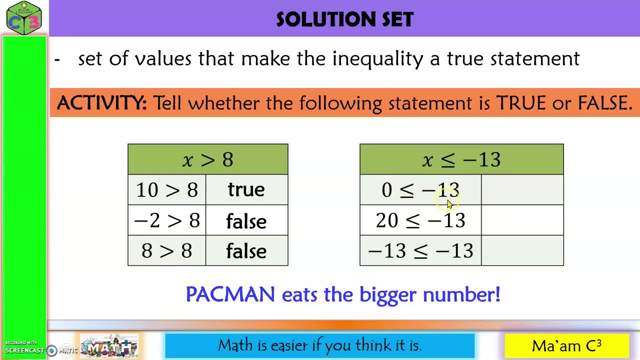 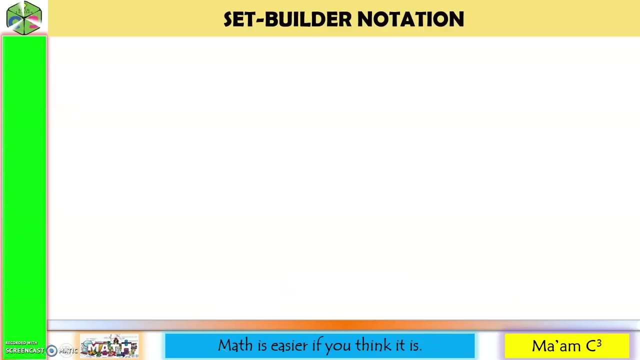 Pac-Man is going to eat negative 13.. Is negative 13 greater than 0?? False. Pac-Man is going to eat negative 13.. Is negative 13 greater than 20? No- False. Here we have the same number and because of or equal to. here this is true. One way of writing. 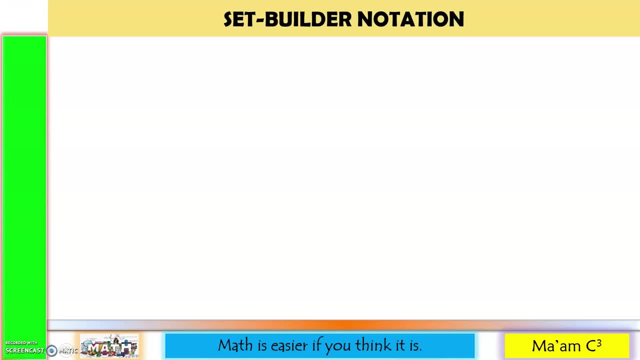 the solution set of an inequality is through set builder notation. This describes the elements of a set instead of listing the elements. It looks like this: The braces is red as the set. of This x here is read as all x. This vertical line here is read as such that. 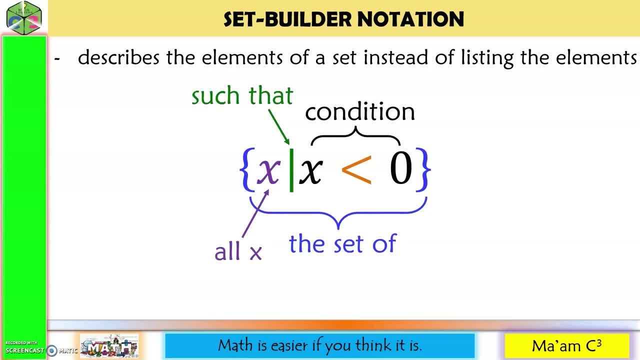 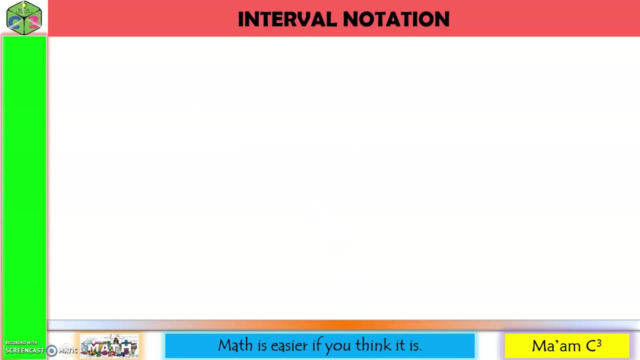 And this portion is the condition. The condition contains the inequality. If we are going to read this, this is read as the set of all x, such that x is less than 0.. Another way of writing a solution set is through interval notation. 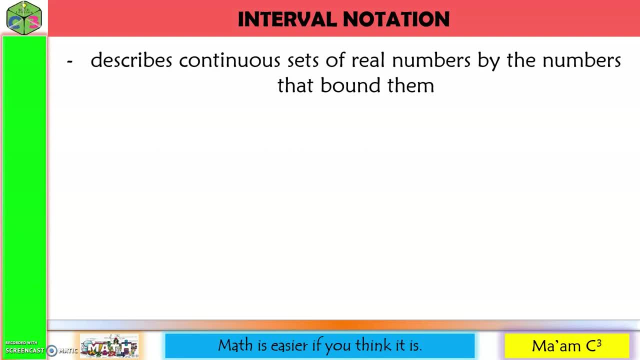 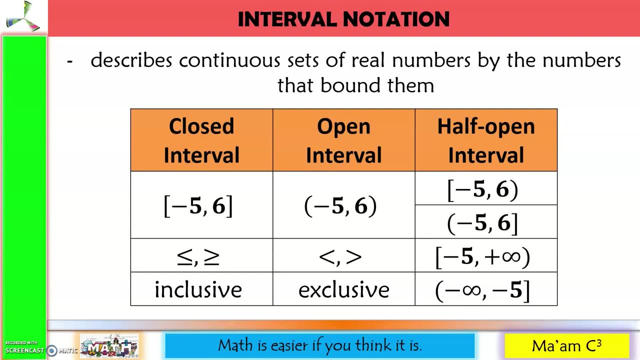 This describes continuous sets of real numbers by the numbers that bound them. We have three types: Close interval, open interval, half open or half closed interval. These are what we call boundaries. This is the lower boundary and this one is the upper boundary. Now for closed. 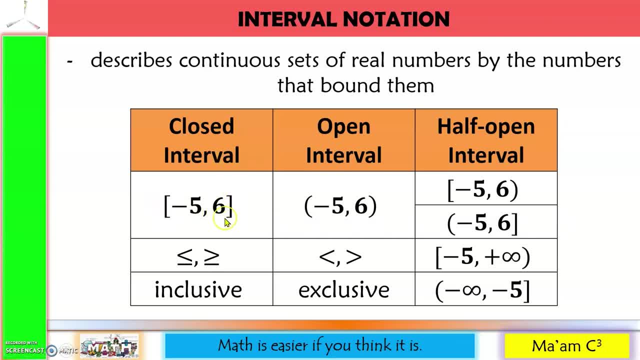 interval. the symbols used are brackets. This corresponds to less than or equal to, and greater than or equal to. This is inclusive, meaning the exact value negative. 5 and 6 are included in the solution set For open interval. the symbol used is a pair of parentheses. This corresponds to less. 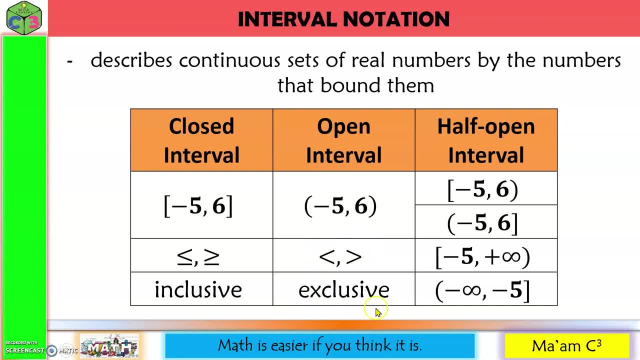 than or greater than. This is exclusive, meaning the exact value. negative 5 and 6 are not included in the solution set For the half open interval. negative 5 is included because we have a bracket here, and 6 is not included because we have a parenthesis here. For this one, negative 5 is. 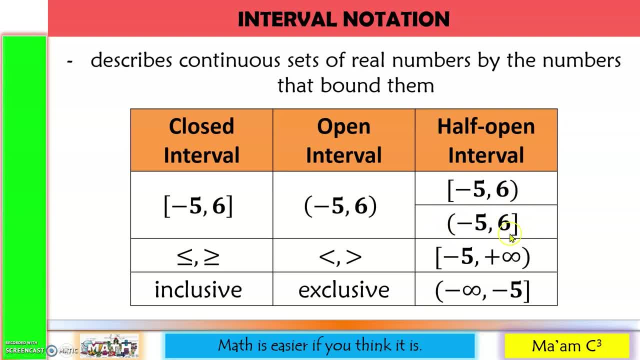 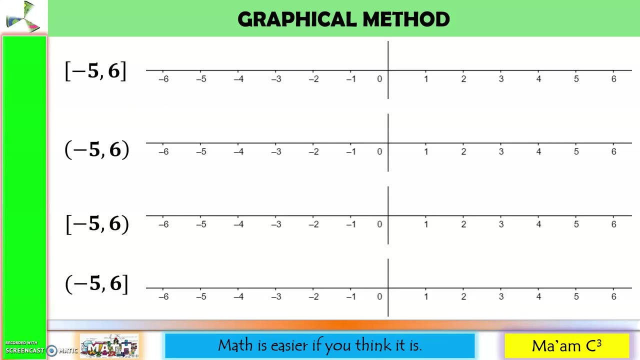 not included and 6 is included. If an interval has no upper or lower bound, the negative infinity and positive infinity are used. Infinity is always used with a parenthesis because infinity is not a specific number that can be included in a set. Another way of writing a solution set. 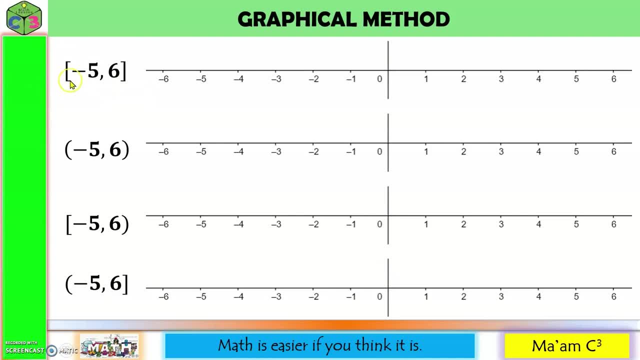 is through graphical method, First example. so these are our boundaries. Negative 5 and 6 are both included because we have brackets here, So let us locate negative 5 in the number line, since this is included in graphical method. we make use of shaded circle Sometimes in other books. 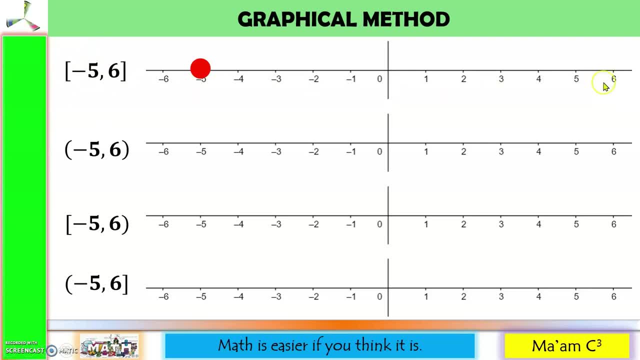 they also use brackets, So let us locate 6, it's here also included. so shaded circle. Since these two are boundaries, then the numbers between them are also included. Next one negative: 5 and 6, but this time they are not included. 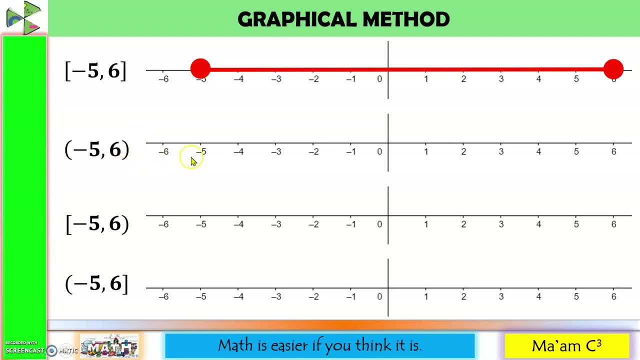 Since we have parentheses here, So let us locate negative 5.. If it is not included, we make use of hollow or empty circle. In other books they also use parentheses. Let us locate 6,, also not included. so empty or hollow circle And the numbers between them are included. So what is the difference? 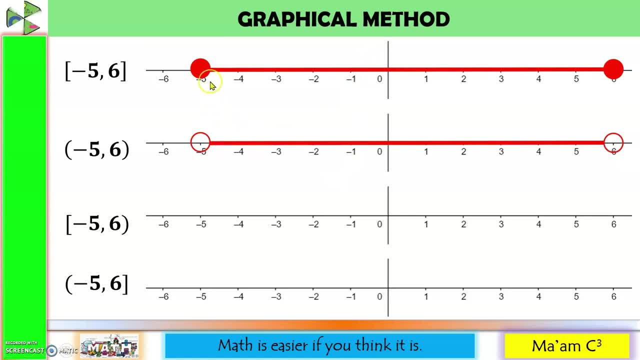 between these two. In number 1, negative 5 is included. So let us locate negative. 5 and 6 are included In number 1, the exact number, negative 5 and 6 are included in the solution set, While in 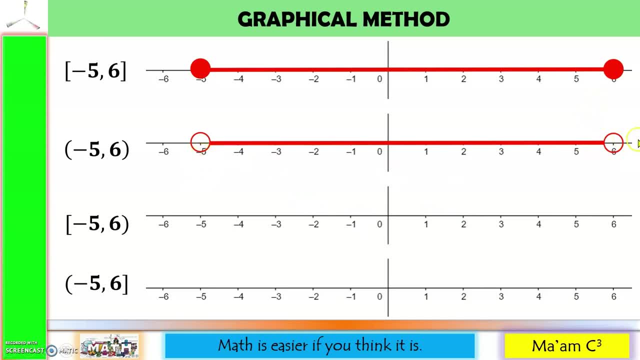 number 2, the exact numbers negative 5 and 6 are not included in the solution set, But the numbers close to them, like negative 4.5, negative 4.7, negative 4.9999, are included in here: 5.5, 5.6. 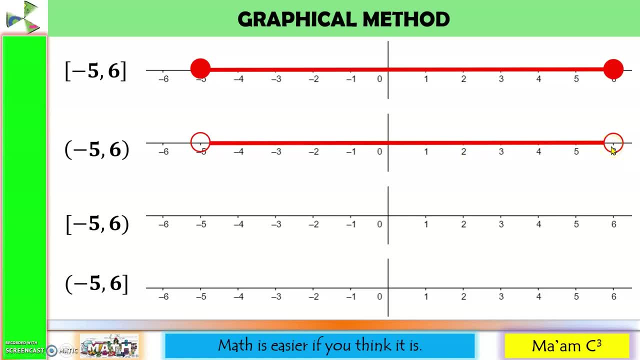 5.7, 5.8, 5.9999 are included. the only numbers that are not included are the exact value of negative five and six, number three. negative five is included because we have bracket here, so shaded circle. six is not included because we have parenthesis, so empty circle, and the numbers. 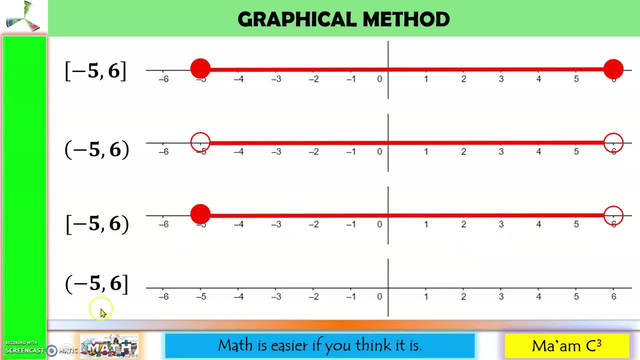 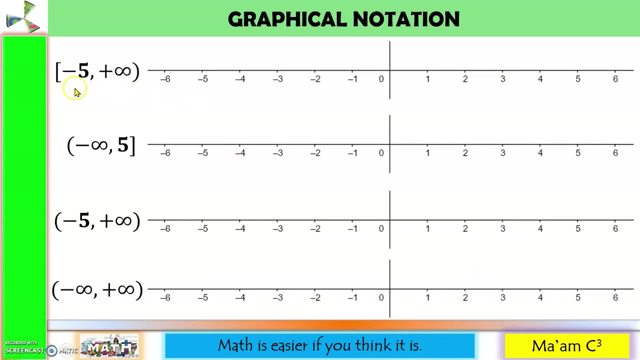 between them are included. next one: negative five, not included, empty circle. six included, so we have shaded circle and the numbers between them. let us continue here. we have negative five included, so negative five, shaded circle. and then going to positive infinity: positive infinity is on the right, so we'll make use of a line with arrowhead pointing to the right. 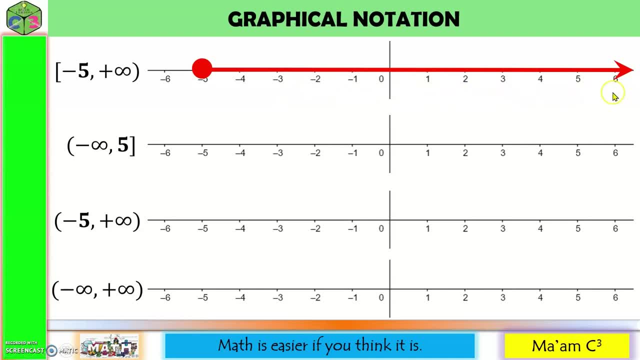 so this means it will go infinitely to the right without bound, to positive infinity. next one, let me graph first: five included, so five included, so shaded circle. and then it is started from negative infinity. so let's make use of a line with arrow head at the end, pointing to the left, meaning this will go to the left without bound. 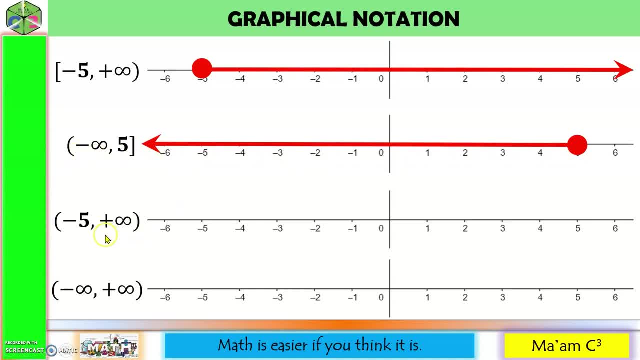 going to negative infinity. this one negative, five not included. so open circle. and then going to the right, because it is positive infinity. Last one: negative infinity to positive infinity. So align with two arrowheads at the end, One is pointing to the left, going to negative infinity. 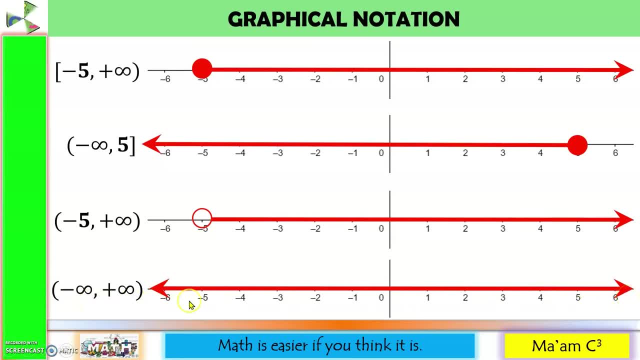 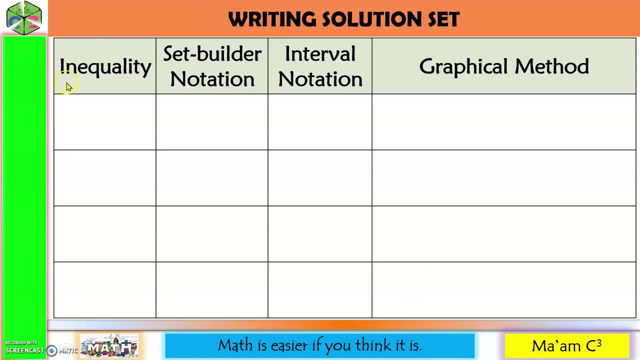 and one is pointing to the right, going to positive infinity. This time, let us write the solution set in three different ways. given an inequality Number one, x is greater than negative one. For the set builder notation, we'll start with x, such that x is greater than negative one. 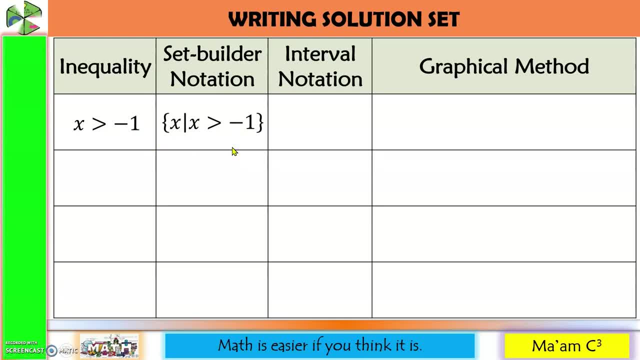 Do not forget to enclose this with braces For the interval notation. remember that we have boundaries, lower and upper boundaries. So we have: x is greater than negative one, So the lower boundary here is negative one. And then comma, upper boundary greater than. 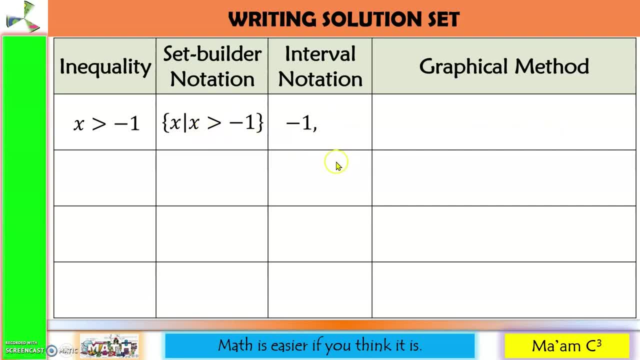 So it means going to the right, going to positive infinity. Negative one is not included, since there is no or equal to. So we are going to use parentheses In infinity. we always use parentheses For the graphical method. let us draw the number line. 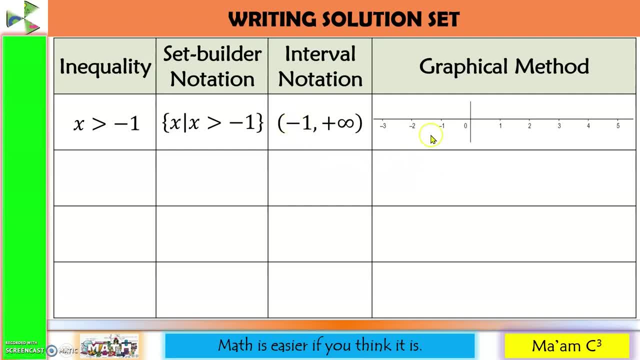 and then negative one, not included, So negative one, hollow circle, And then going to positive. infinity means going to the right, An arrowhead that points going to the right. Number two, x, is less than three, So x, such that x is less than three. 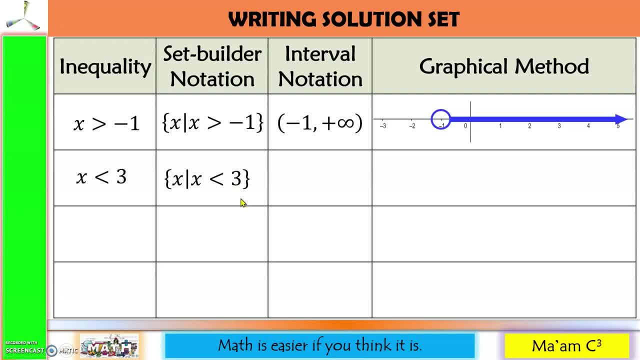 Don't forget enclose this with braces. Let me graph this one first. So number two: x is less than three Number line, And then three not included. There is no or equal to So three empty circle. 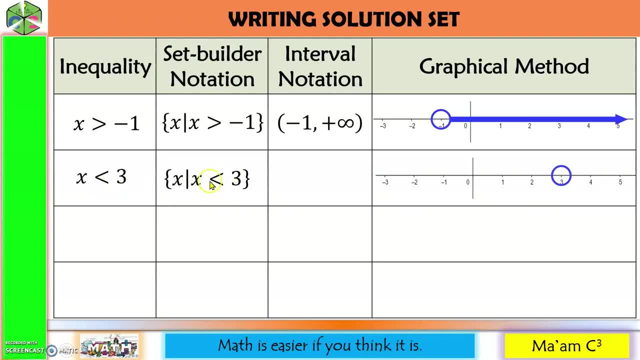 And then going to the left, because less than three Values of x that are less than three, So two, one zero, and going to the left Meaning going to negative infinity. If you have the graph, it is easier to create the interval notation. 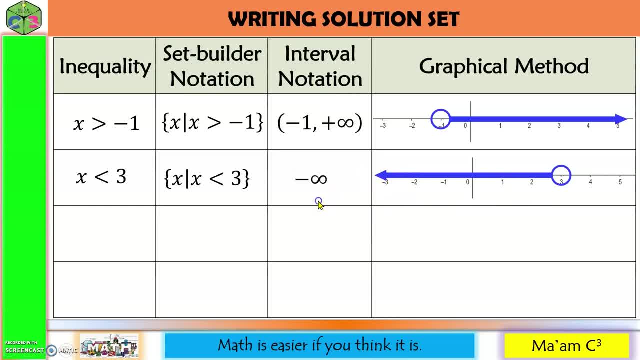 So we'll start with. this is started from negative infinity comma up to positive three, Again for infinity. we always use parentheses, And then three is not included, because this is an empty circle. So also parentheses. Next one: x is less than or equal to negative two. 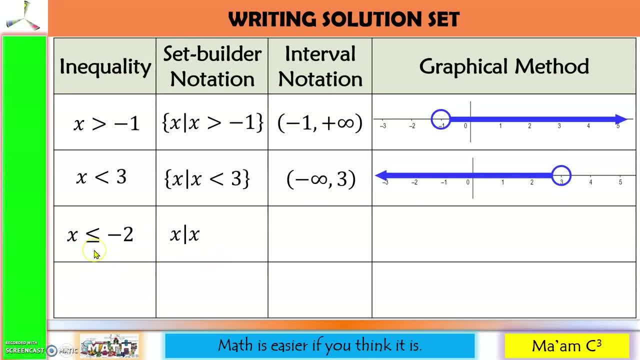 X, such that x is less than or equal to negative three. So negative two Enclose with braces. Again, I'll graph this one first. I'll start with negative two, Negative two included. So from negative two I'll make use of shaded circle. 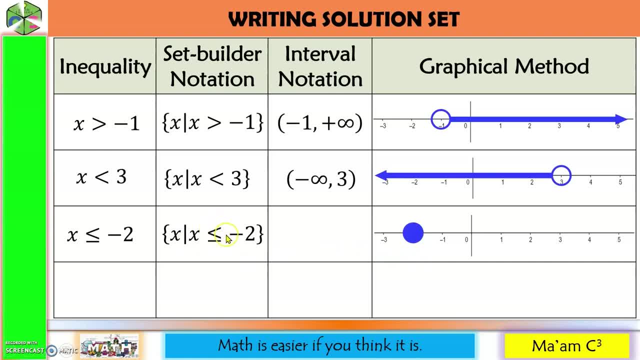 And then values of x that is less than negative two. Those values are negative three. negative four. negative five, going to the left. Now I can write this So I can easily set up the interval notation. This is from negative infinity comma up to negative two. 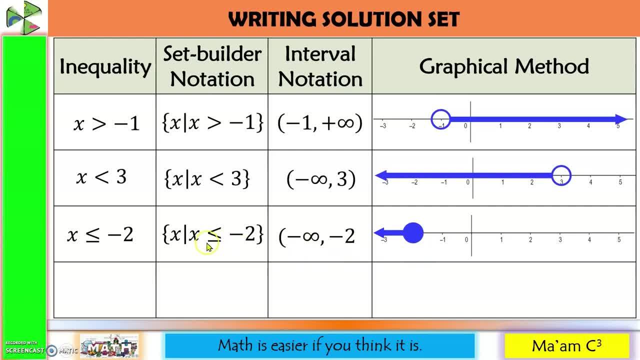 Infinity parentheses. negative two is included because there is or equal to, So we'll make use of bracket Last one: x is greater than or equal to zero X, such that x is greater than or equal to zero X, such that x is greater than or equal to zero. 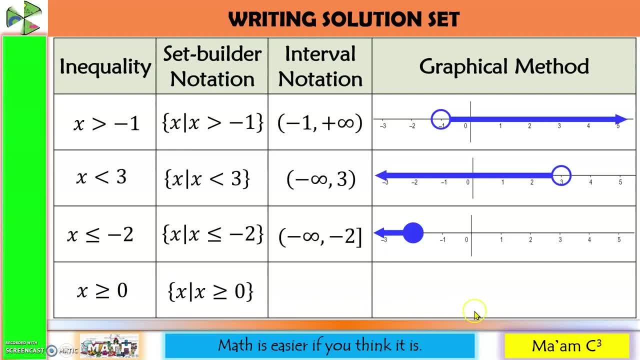 Enclose with braces. I'll graph this one first. I'll start with zero or equal to So, in zero shaded circle, And then going to the right, because x is greater than Values of x that are greater than zero: One, two, three, four, five. going to the right. 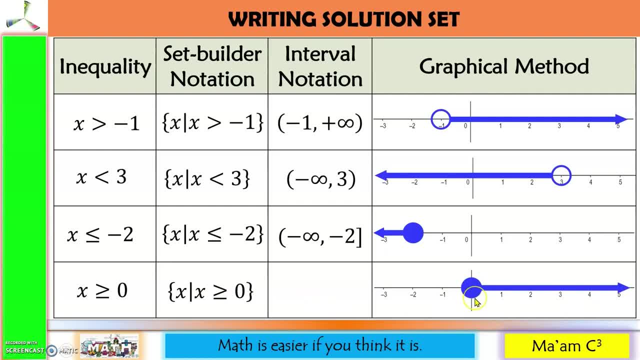 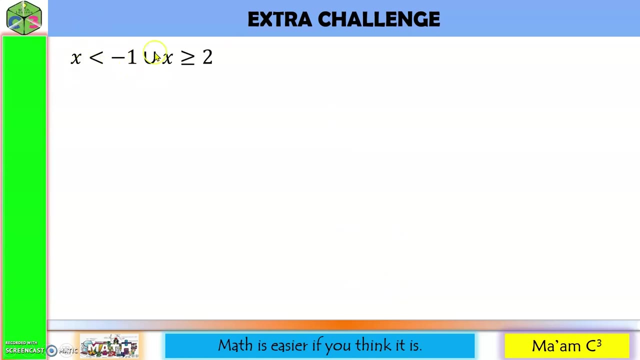 So the interval notation is started from zero, Zero comma going to the right positive infinity, Zero is included, So we'll make use of bracket Infinity. always use parentheses. Let us do extra challenge. Number one: x is less than negative one union. 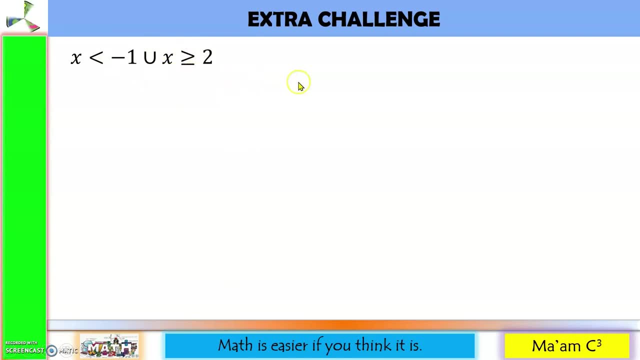 X is greater than or equal to two. For the set builder notation, we simply have to copy that X such that x is: X is less than negative one union with x greater than or equal to two. Let us graph. Let us start with negative one not included. 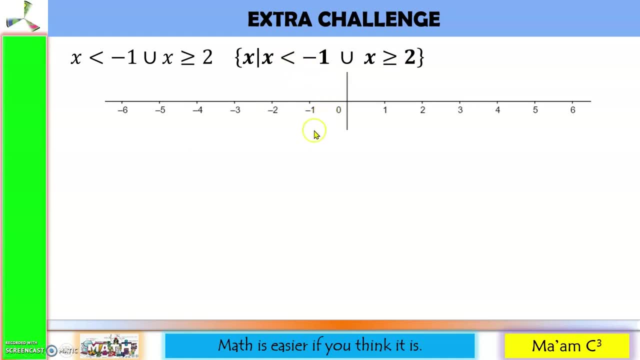 There is no or equal to. So in negative one empty circle, X is less than Values of x that are less than negative one. Those are negative two negative three negative four going to the left, This one, X, is greater than or equal to two. 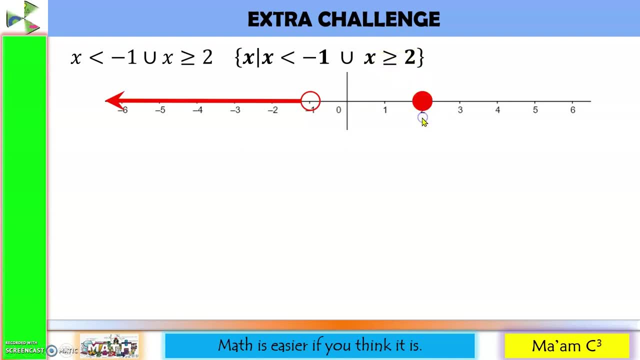 So in two there is or equal to shaded circle Greater than two. Those are three, four, five, six, meaning going to the right. For the interval notation, it started from negative infinity up to negative one not included. 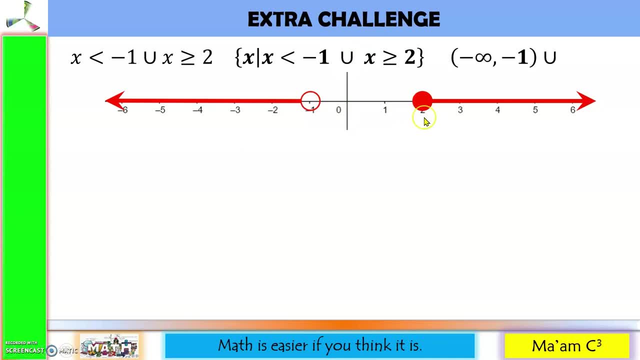 Union started again at two, going to positive infinity. Two is included, so bracket in two. Another example for the set builder, notation x, such that x is less than three, but greater than or equal to negative three. Let us graph: 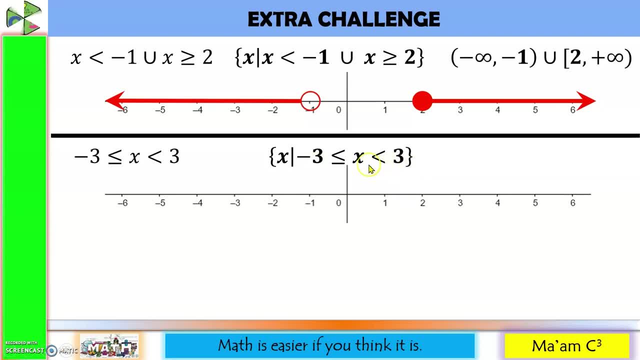 Let us start with the right side. Three not included, so open circle: X less than. So values of x that are less than three. Negative two, one zero. going to the left. Now for here. negative three is less than or equal to x, meaning x is greater than or equal to negative three. 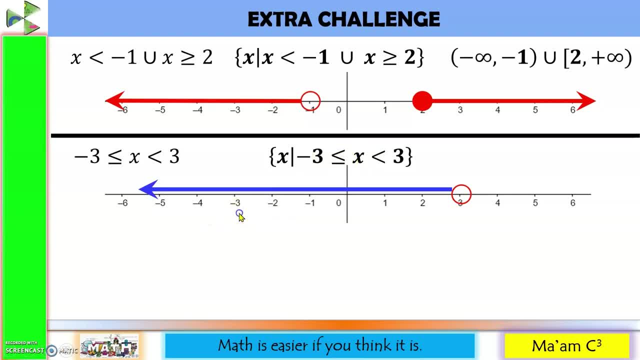 So negative three there is, or equal to shaded circle, Greater than negative three. those are negative two, negative one, zero, going to the right. Next we have to get the intersection of x, The intersection of these two, and those are from negative three to positive three. 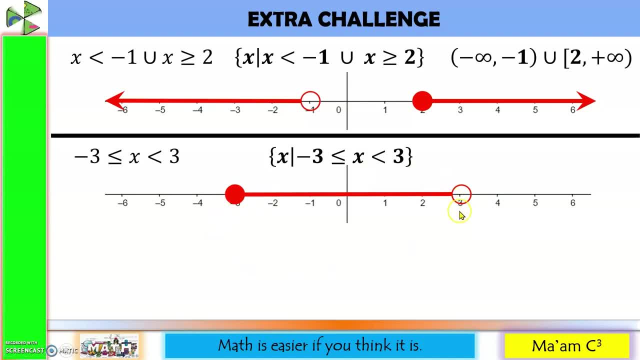 Interval notation: negative three included. positive three not included bracket and parenthesis. Last one: x is not equal to zero. Set builder notation x such that x is not equal to zero. Let us graph In the number line: only zero is not included. 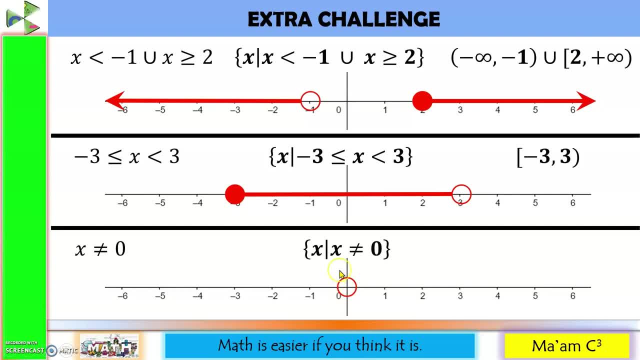 In the solution set. so empty circle on zero and then going to the left and going to the right. For the interval notation from negative infinity up to zero not included. union with started at zero to positive infinity. This means only zero is not included in the solution set. 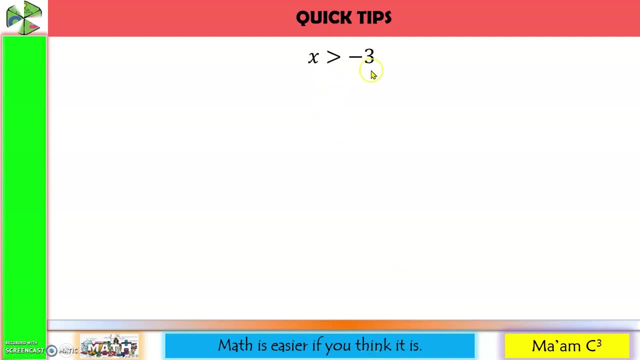 Some questions, Big tips. If you are given x is greater than negative three, it is very easy to graph. You start with negative three, since there is no or equal to, so we have empty circle And then look at the inequality symbol. 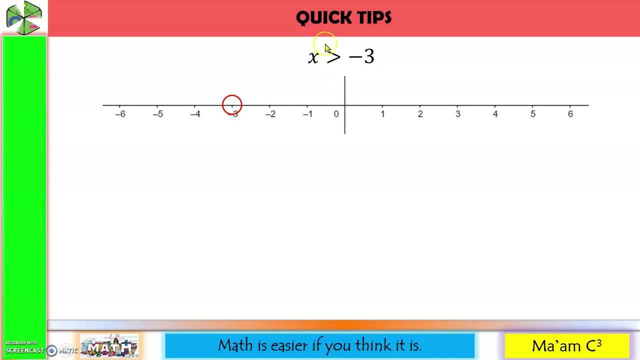 Look where the inequality symbol points you, And this one points to the right. So you go to the right, That's it. But what if you are given like this: Are you going to start at negative three And then follow where the inequality symbol points you? 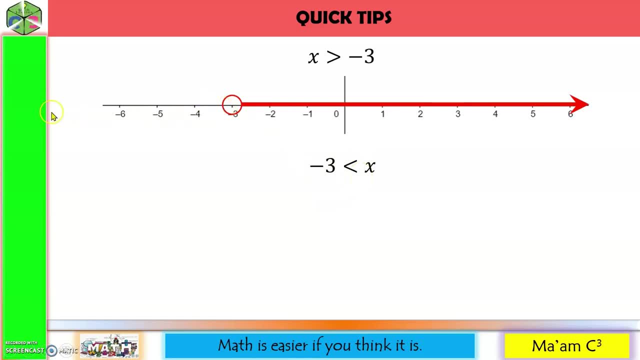 So this means going to the left? then that would be wrong, Because if the given is like this, we have to start reading from the variable side And when we read, we read the inequality symbol in the opposite direction. So if this is less than you're going to read it as greater than. 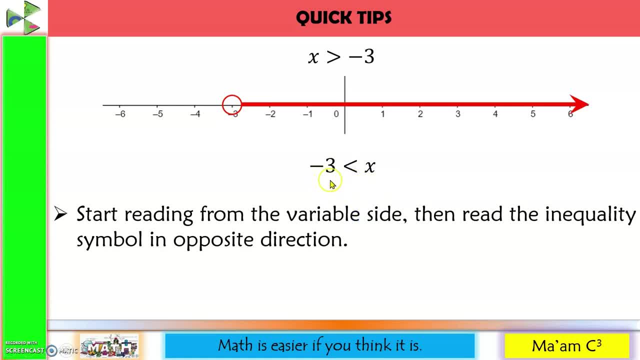 So this is x is greater than negative three, Then it will be like this, So it will be easier to graph. So my tip is, if you want to graph the inequality in an easy way, make sure to write the variable on the left side. 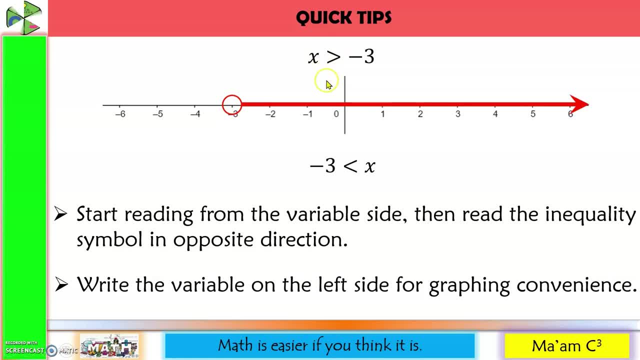 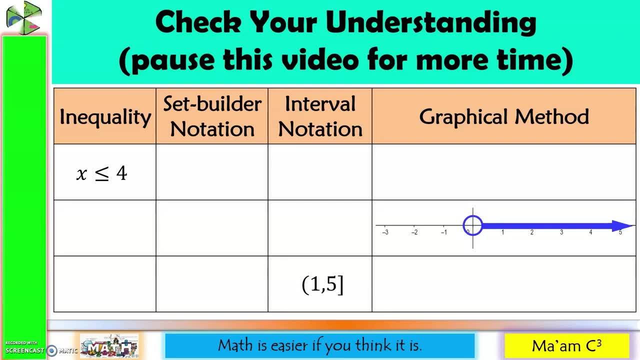 From then, you will only follow where the inequality symbol points you. Now it is time to check your understanding. Pause this video for more time. Let us answer Number one. x is less than or equal to four. Set builder notation x such that x is less than or equal to four.